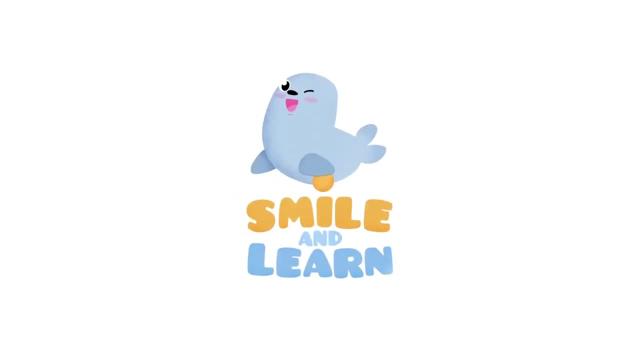 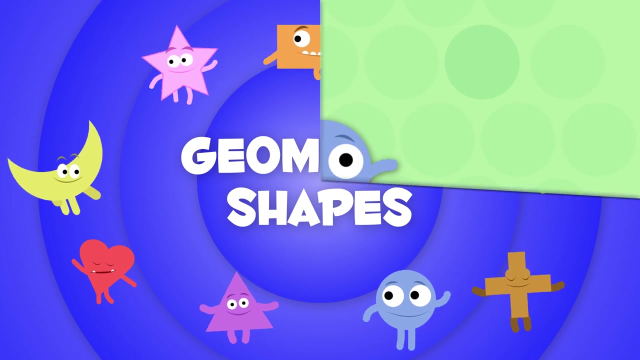 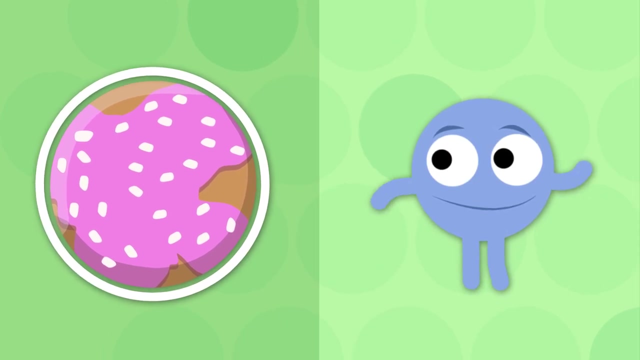 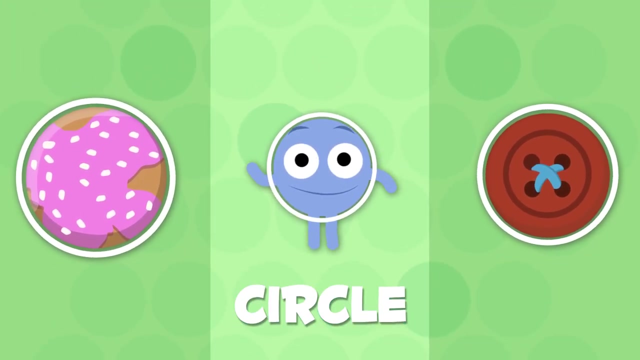 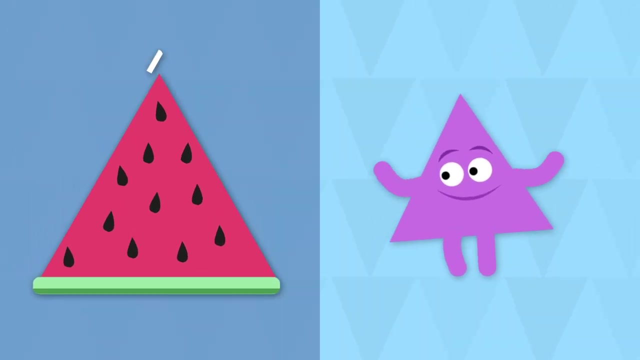 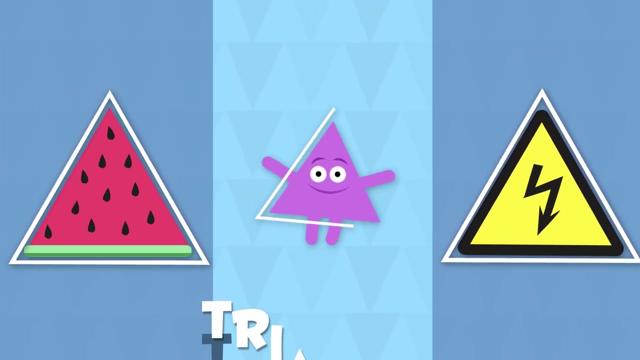 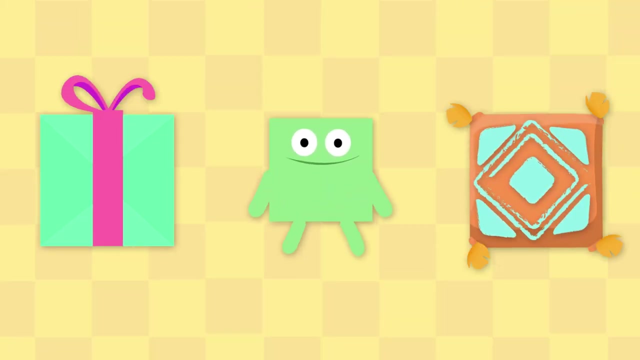 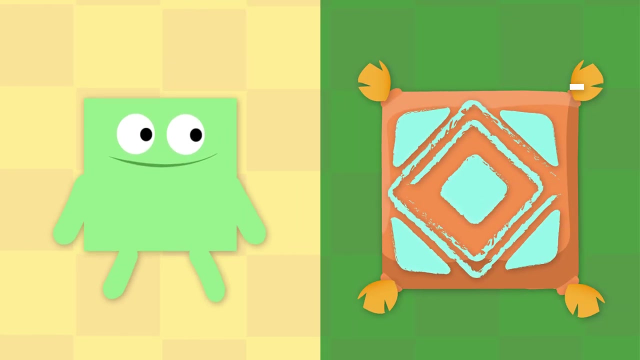 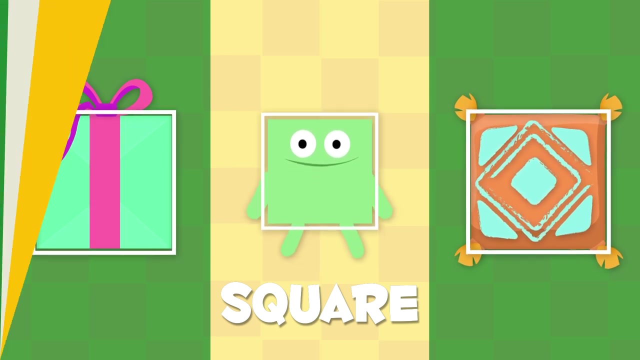 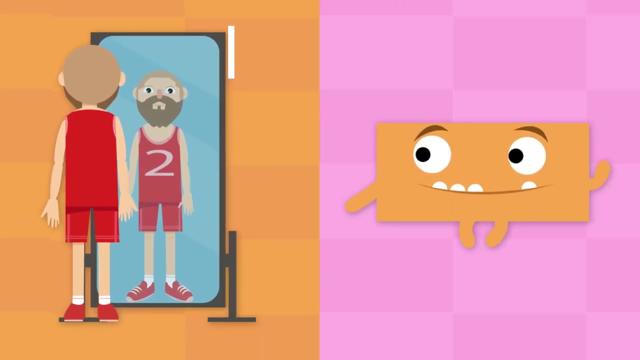 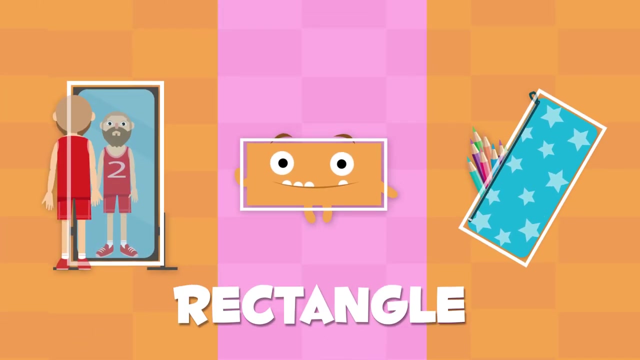 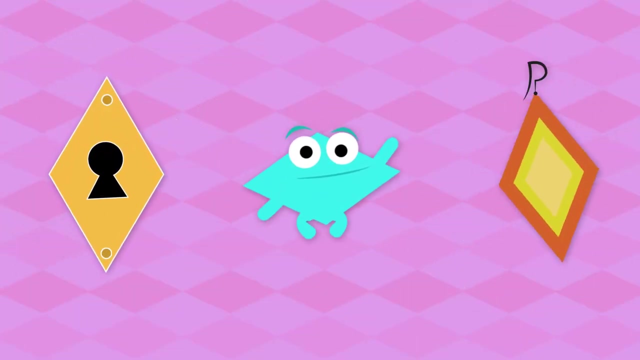 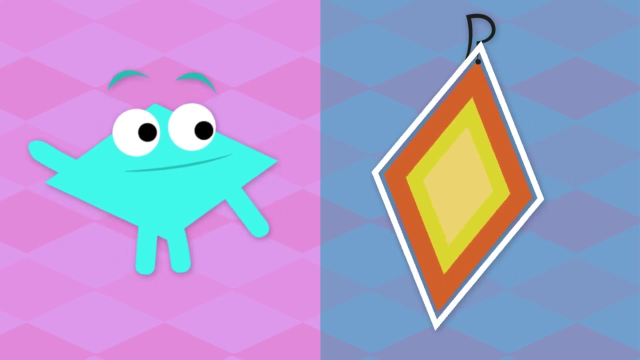 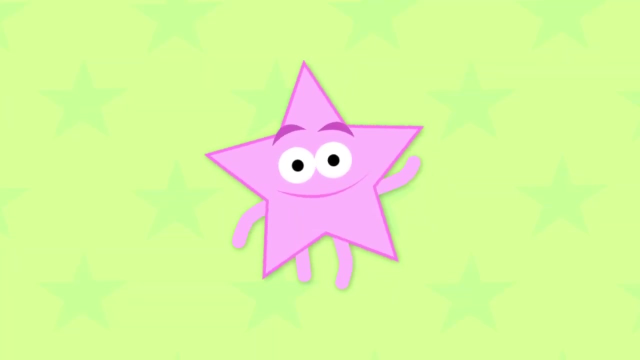 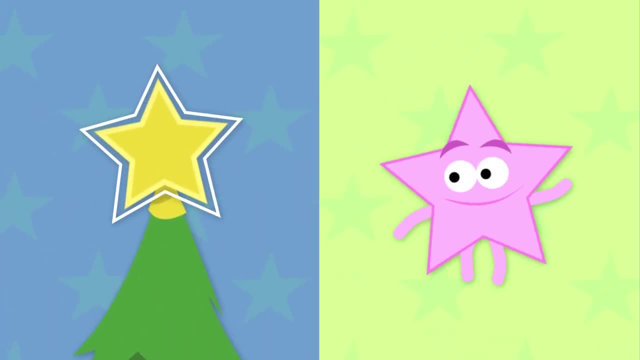 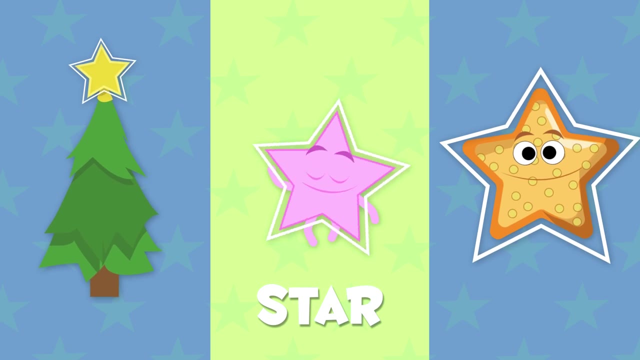 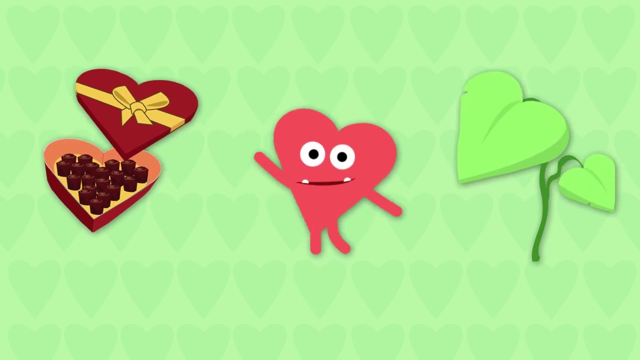 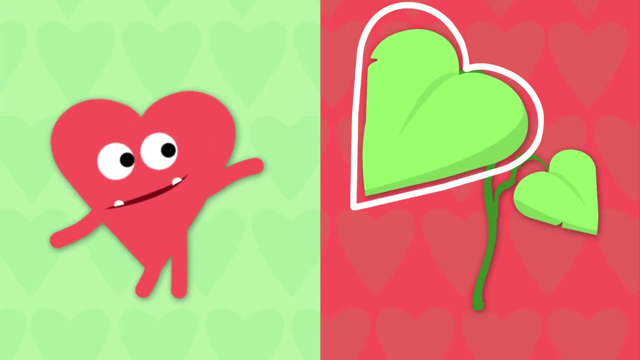 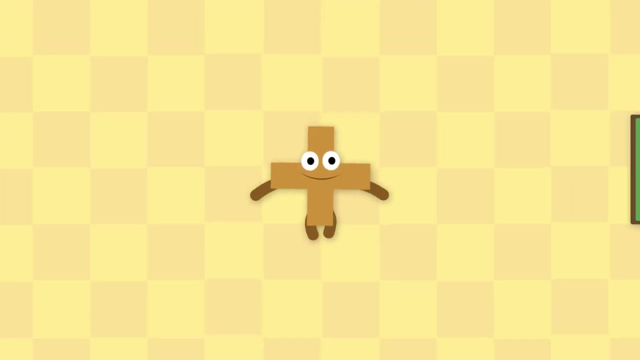 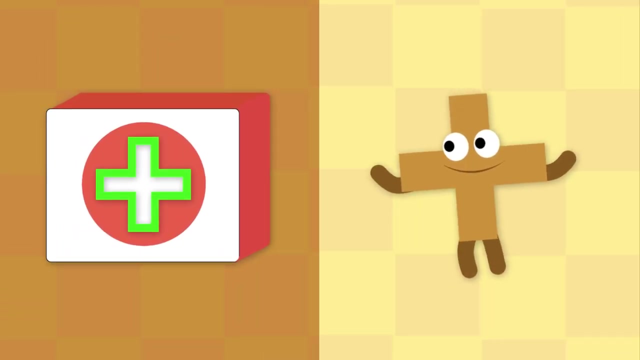 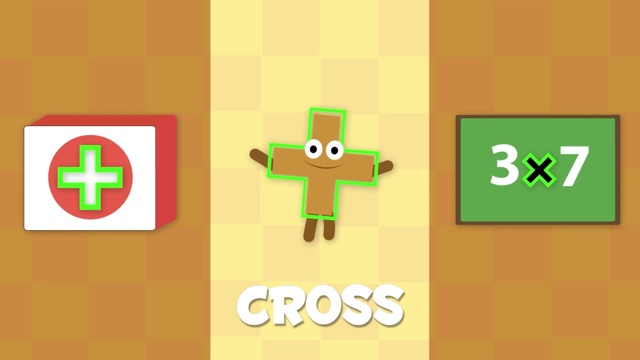 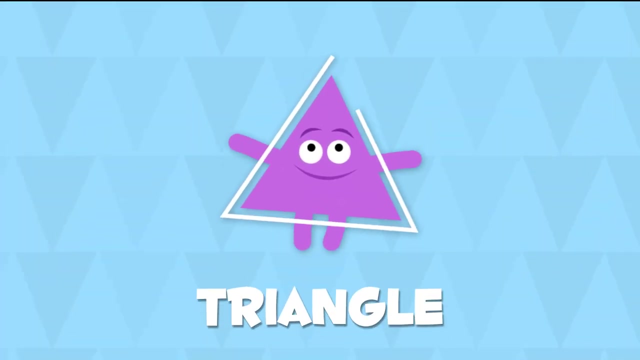 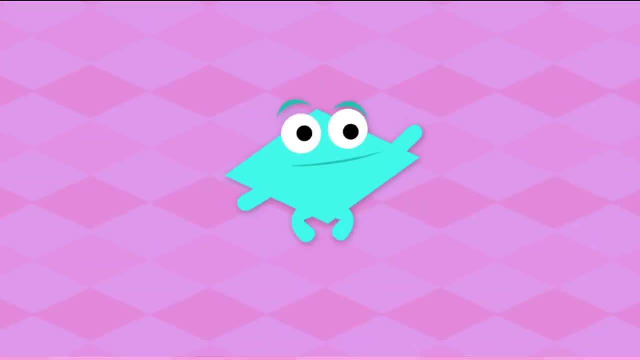 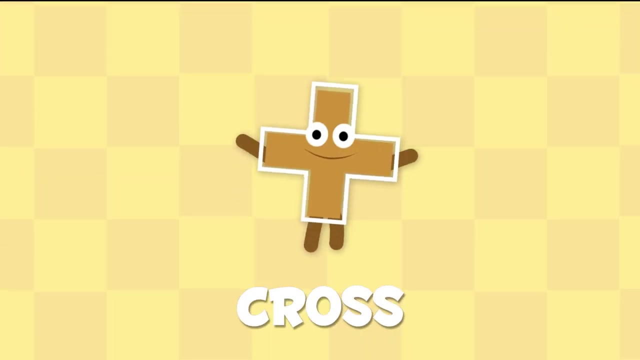 Rectangle: Diamond Star, Heart Cross. Thank you for watching.